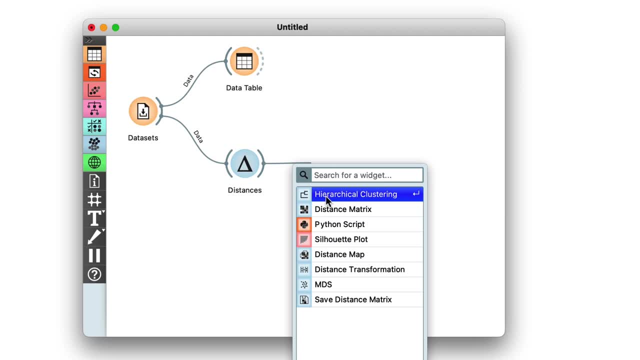 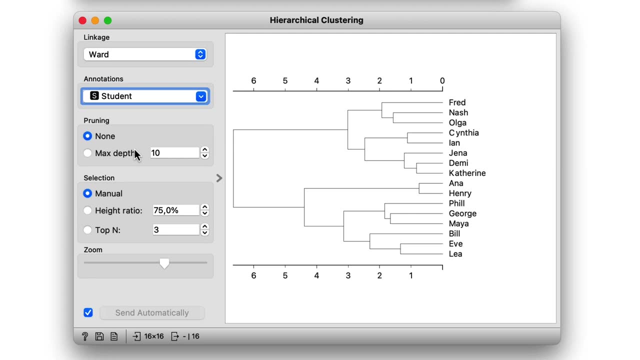 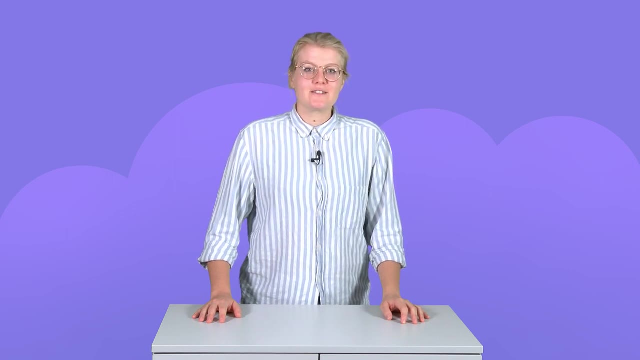 accordingly. Here I will use the word minimum variance method for linkage. This will join clusters so that the points in the resulting cluster are nearest the center. It's a bit more complicated than that, but the idea of word linkage is that the points in the resulting clusters are as close together as possible. 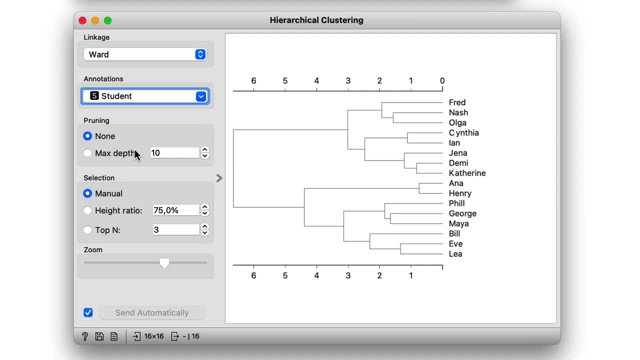 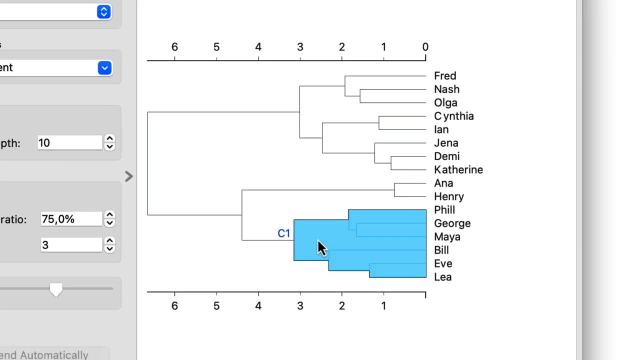 My problem here, however, is not the number of students, but the number of clusters. It's not a clustering algorithm, but how to interpret the resulting clustering structure. Why are Phil, Bill and Leah in the same cluster? What do they have in common? 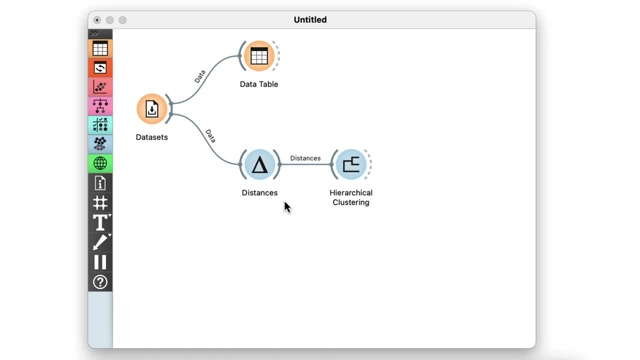 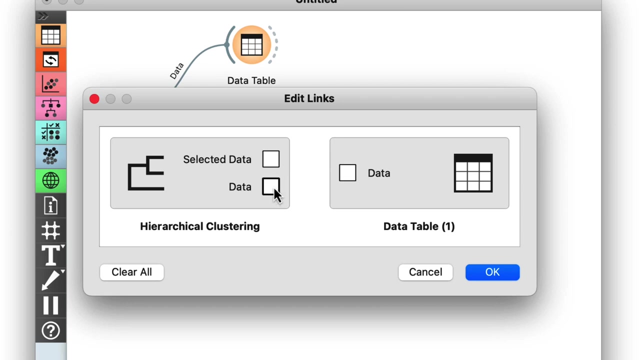 The hierarchical clustering widget emits two signals: selected data as well as the entire data set, with an additional column that indicates the selection. Let me first show this in the data table widget. I have to rewire the connection to the data table. I have to rewire the connection between hierarchical clustering and data table to communicate. 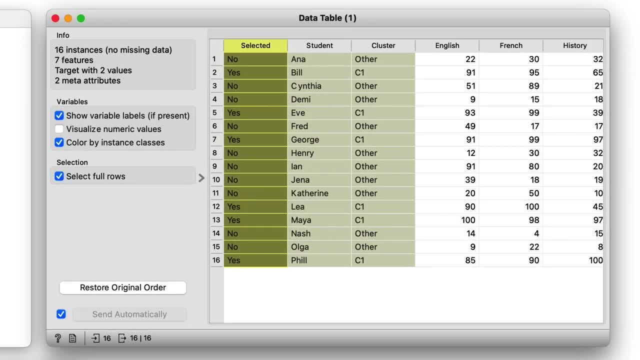 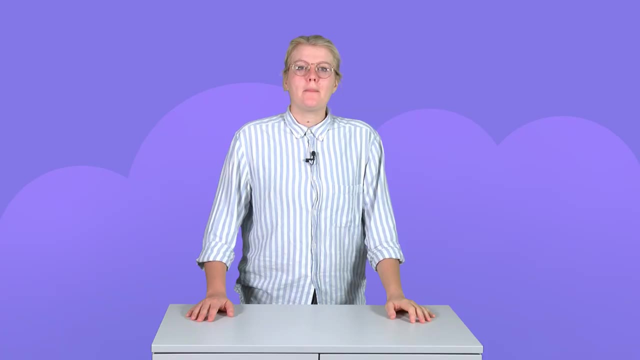 the entire data set: See the selected column in the data table. We would now like to find the features, that is, school subjects, which can differentiate between selected students and students outside the selection. But wait a second, This is something we have already done. 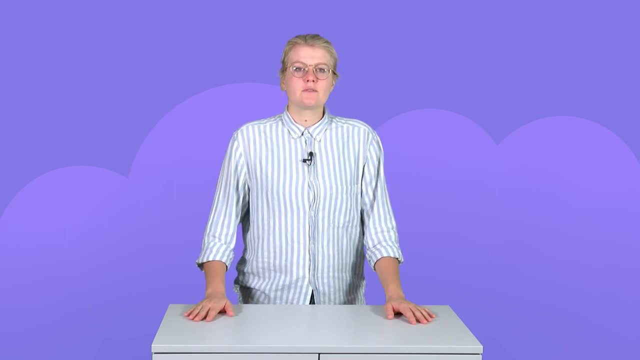 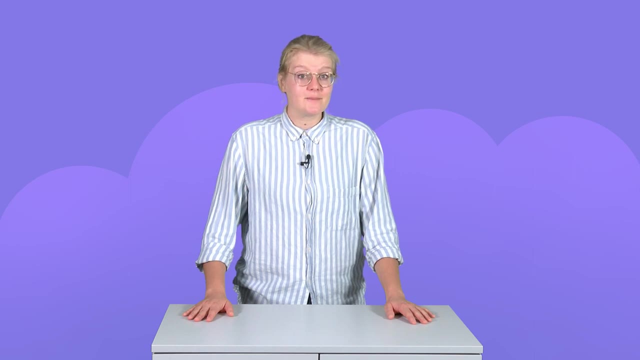 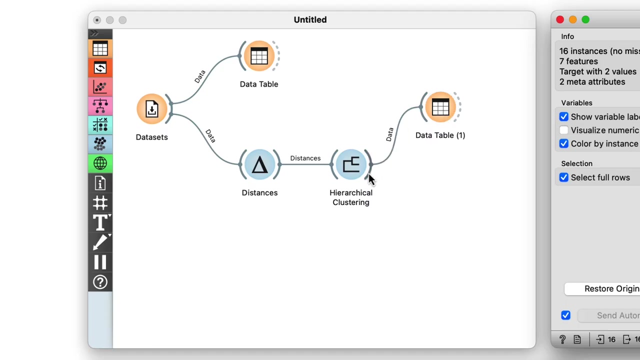 Remember our video on data distribution where we constructed the data table? Yes, we did. This is a workflow that told us which socio-economic features are related to extended life expectancy. Maybe not, but you can always check that out on our channel. The critical part to remember is that we used Boxplot. 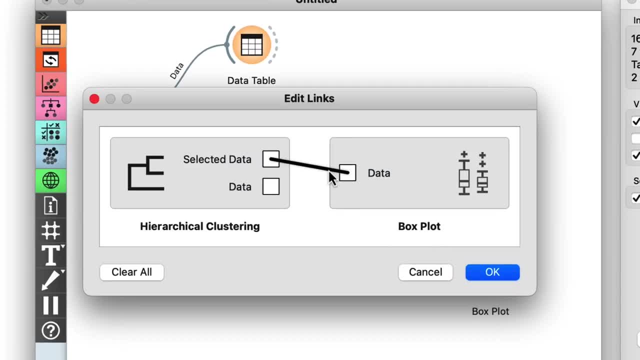 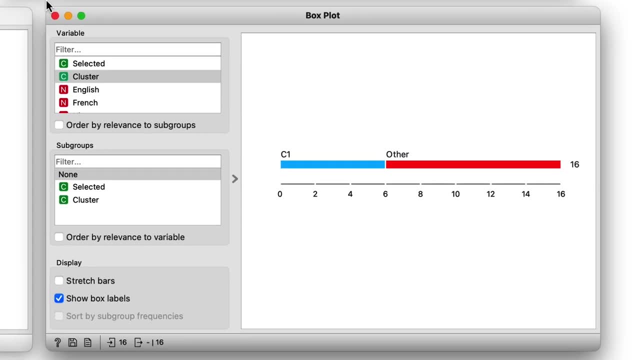 Let me add one to the output of hierarchical clustering and rewire the signal to transfer all the data instead of just a selection In Boxplot. I have to set selected as a subgrouping feature And I also check order by relevance to subgroups. 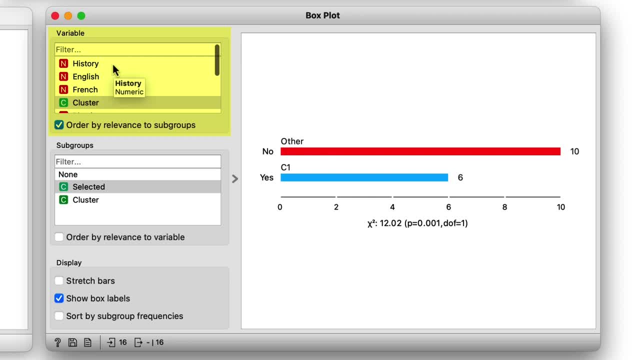 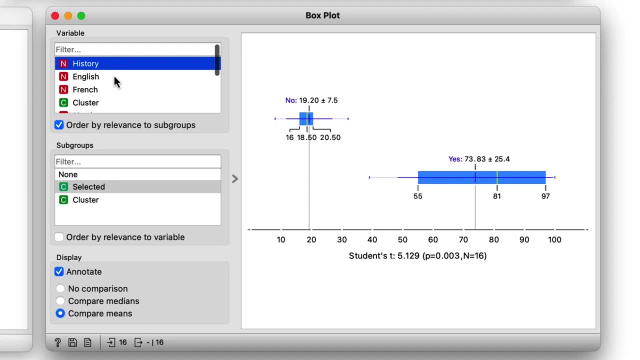 I find history, English and French- at the top of the list of variables. Taking a closer look at history, for example, we can see that Phil George and company perform quite well, their average score being 73. Compare that to the mediocre 19 of everyone else.